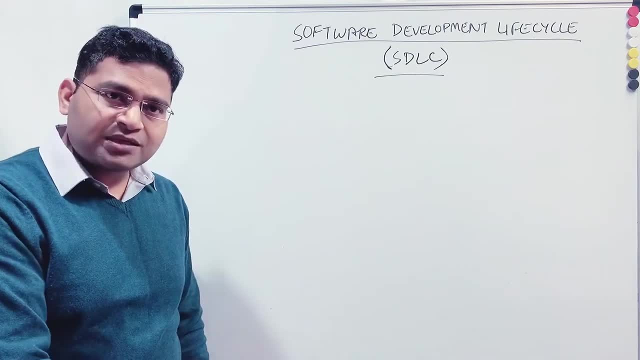 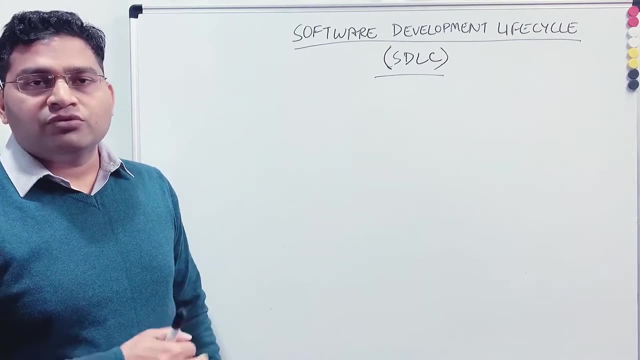 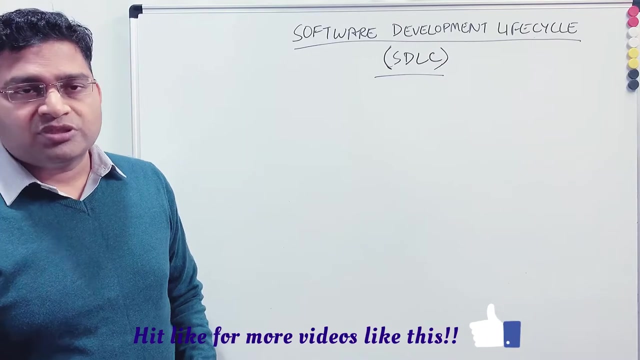 we need to understand if we want to work in the software testing team, we need to also understand what software development lifecycle is and, based on different, you know, approaches, we'll understand how software development lifecycle you know is in different software development approaches. So, for example, waterfall development approach, how SDLC is there. 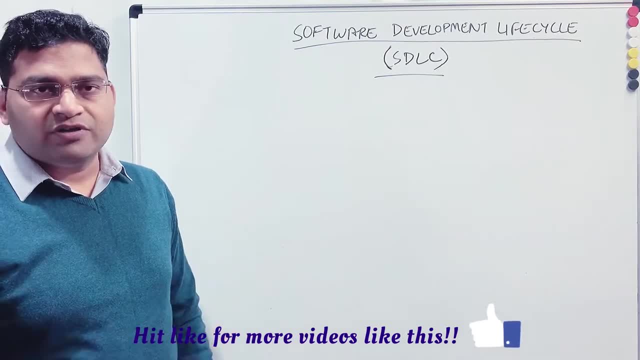 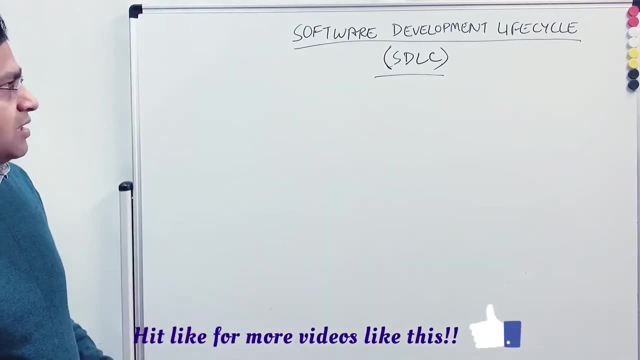 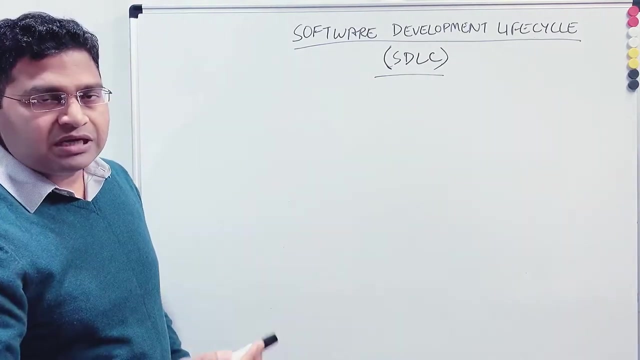 and then, if you are following vModel, how software development lifecycle is in the vModel or in the Agile approach, for example Scrum. So let's start with the software development lifecycle. So here I'll totally cover SDLC and in the next tutorial I'll cover software testing lifecycle, which is 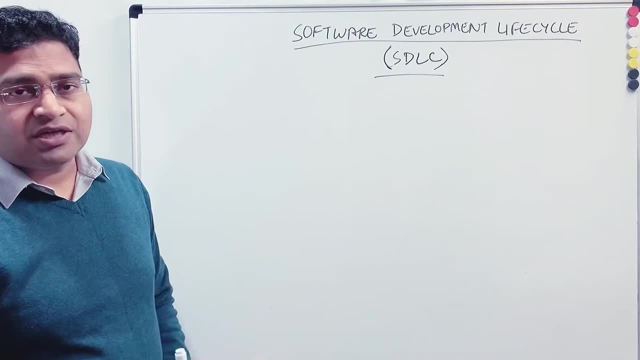 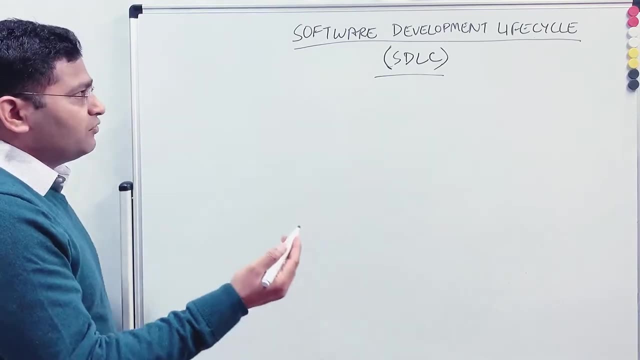 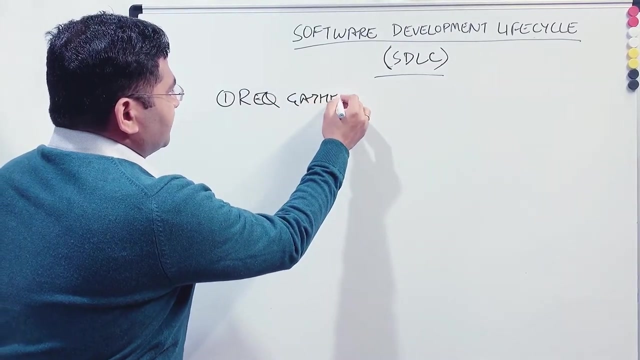 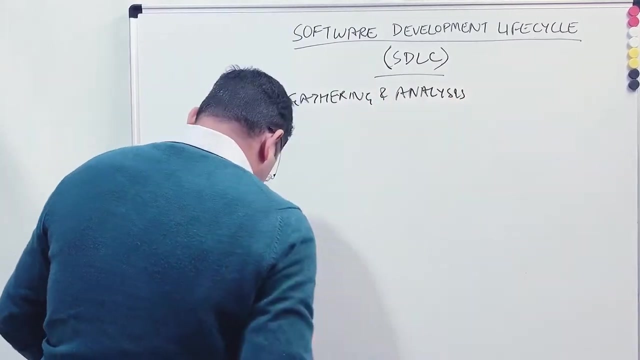 sort of a subset of software development lifecycle. SDLC fits within software development lifecycle. So the first phase in software development lifecycle is the requirement gathering. Okay, so requirement gathering and analysis- Okay. so what does the requirement gathering means? So we'll understand First. 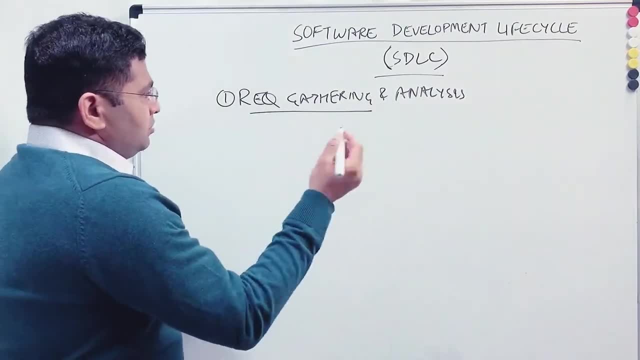 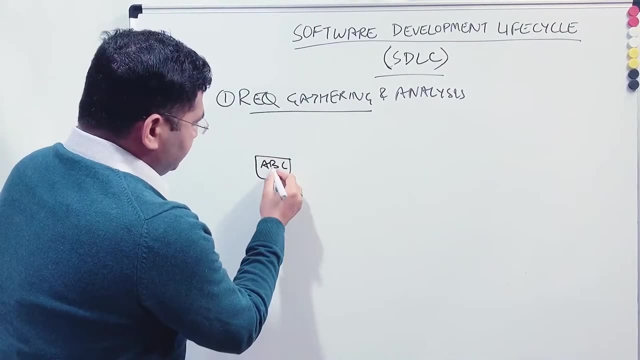 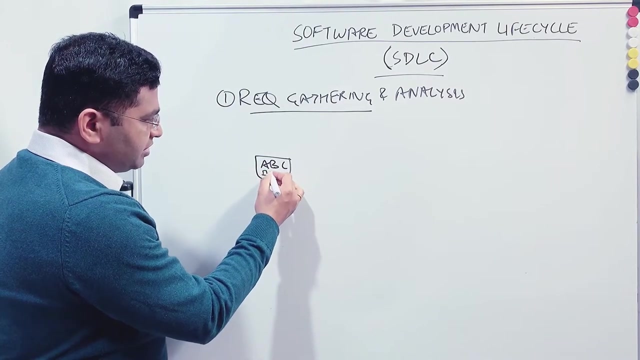 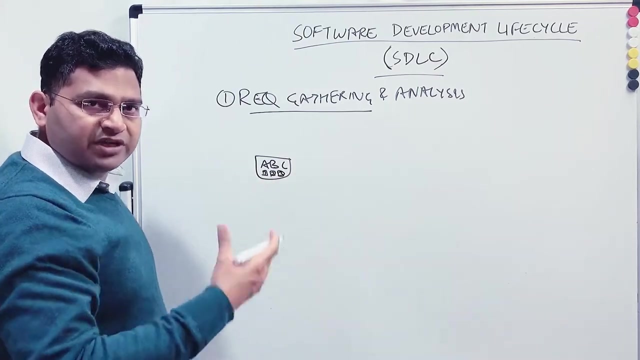 and gathering and then analysis. so say, for example, there is an organization, ABC, and this is the organization which takes the software development project. okay, so you will be, you know, having certain teams there, development teams, so team 1, 2, 3, and these teams basically work on different development project. now any 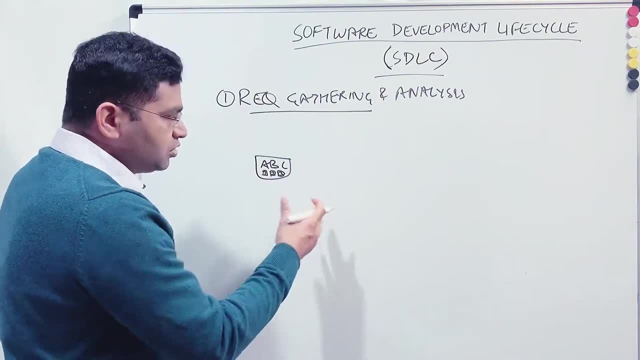 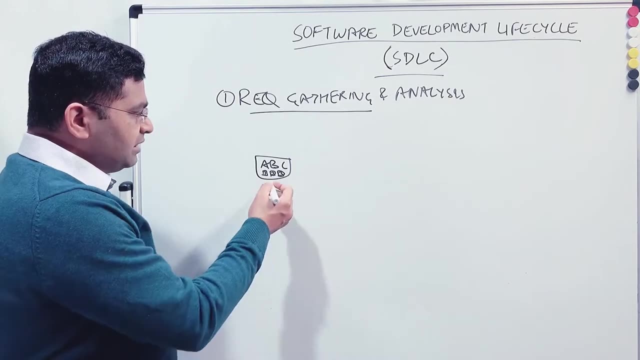 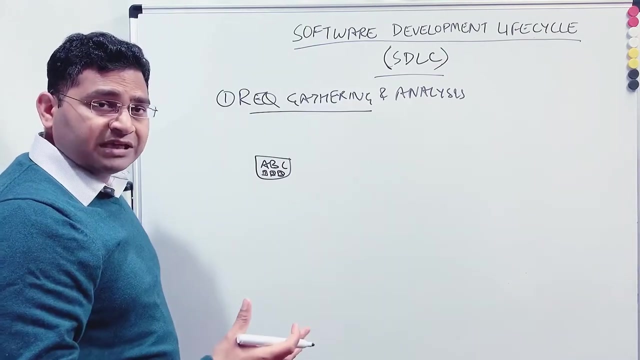 organization or any person who is the customer who wants to build something. say, for example, I am a customer and I want to build an app. okay, so what I'll do is I'll either, if I'm a big organization, I'll, you know, have a tendering, and then I'll announce that I want to build something like this there. 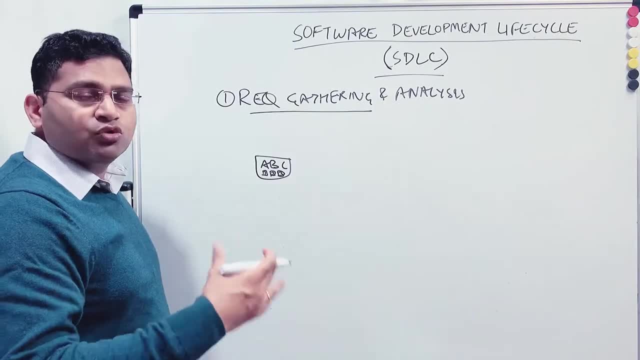 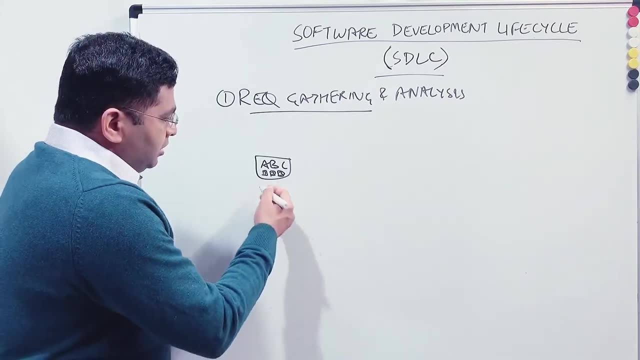 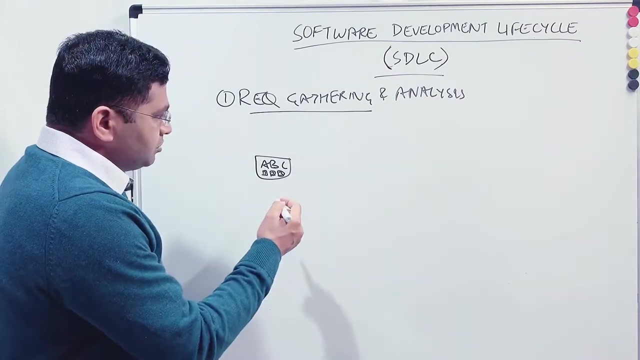 will be multiple organization that will bid and then, based on those bids, I'll choose the organization or the team that I want to give the product. right, so yeah, now, if I want to build an app or a website in the simplest form, okay, so I'll provide some requirements to the organization, right? so what requirement? 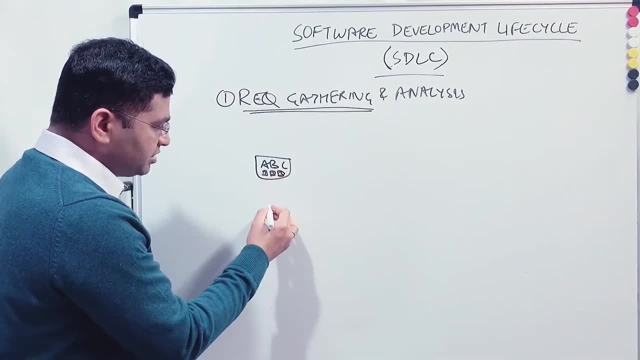 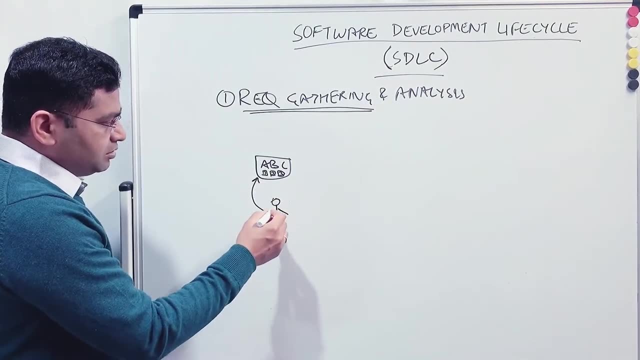 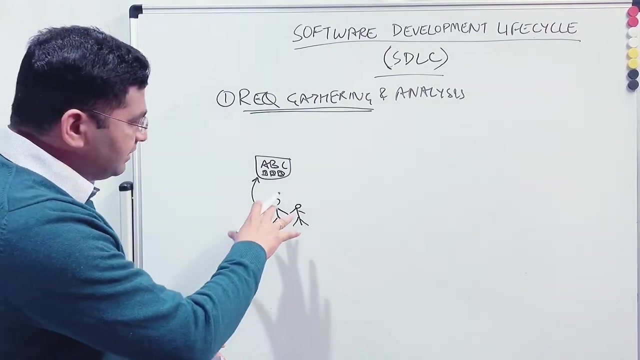 gathering is basically once this ABC organization gets the project and if I am the customer then I will provide the requirements. or, you know, there will be team of people basically in the customer, you know team. so who will provide the requirement to the organization? who wants to build the software right, or who? 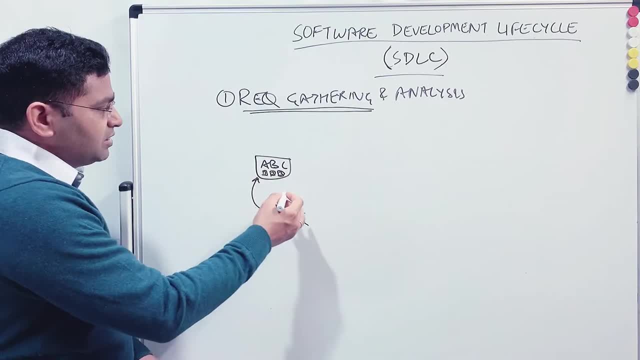 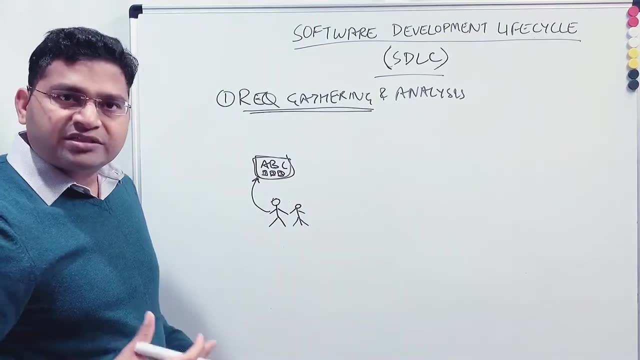 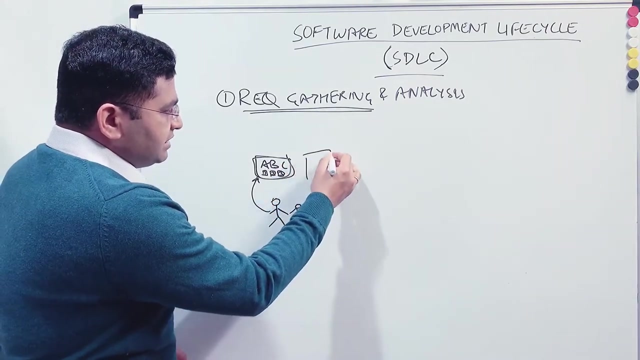 will be building the software for us, so those requirement when gathered by this particular organization is known as requirement gathering. okay, so all the features that I want to be in my app or in my website, I will provide those details and then all the details will be documented. okay, 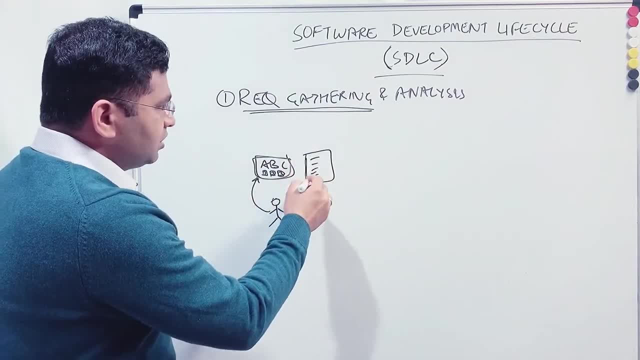 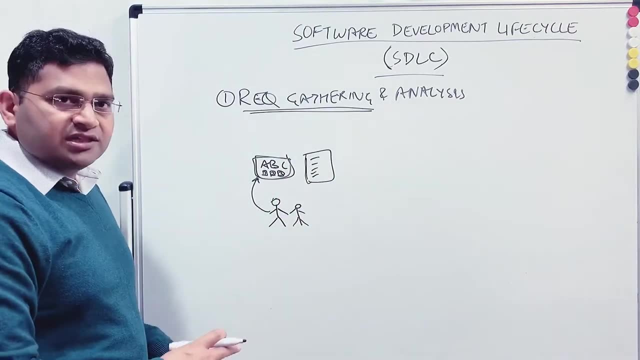 so all the details will be documented and this is what the requirements document is, and this is what the requirements document is In the waterfall approach, this was a lengthy requirements document, but in Agile it's in the form of user stories or epics, basically. 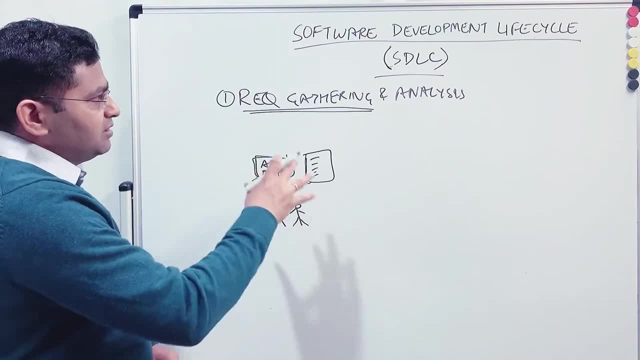 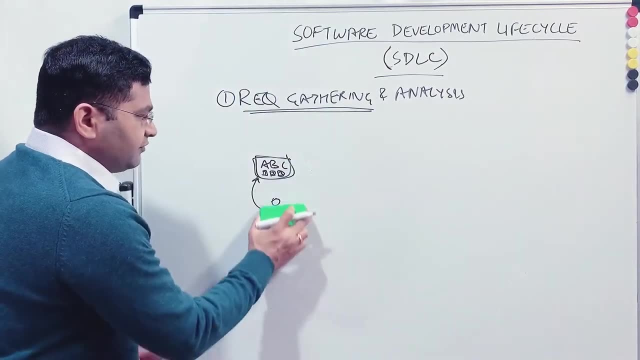 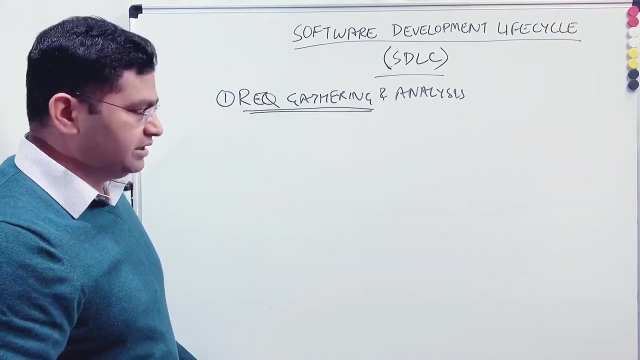 So epic will be the high level user story. That is what captures the high level requirement of the customer. OK, so this is what a requirement gathering phase is: when you gather the requirement about the software, what customer is actually looking for or, in terms of feature, what the customer is looking for into the software or the app that you're trying to build. 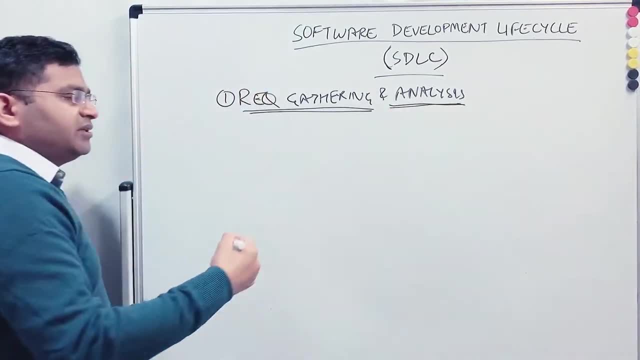 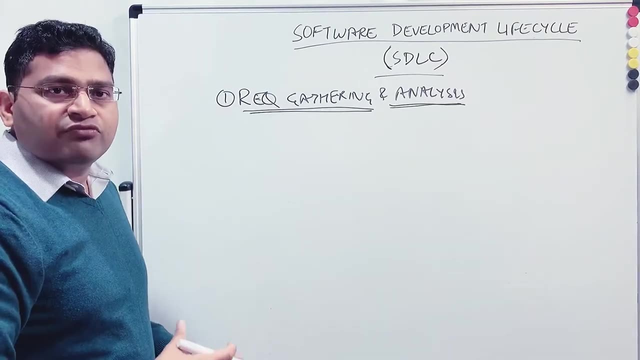 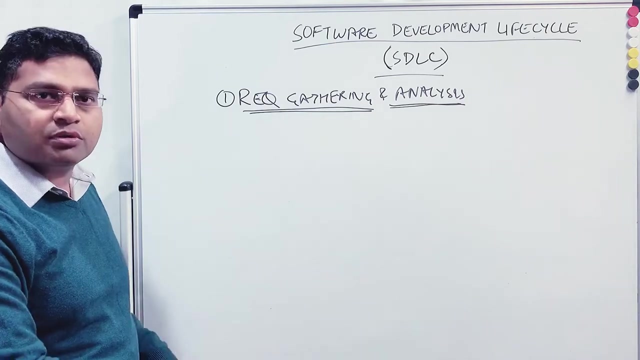 Then the analysis phase is basically: once you gather the requirement, you also analyze the requirement whether those requirements are feasible or not Right. So feasibility analysis is very important. So once the customer provides a certain requirement, there might be some limitations in terms of technology support or any other issues. 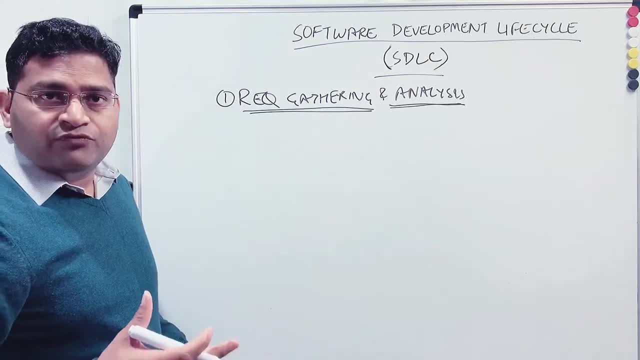 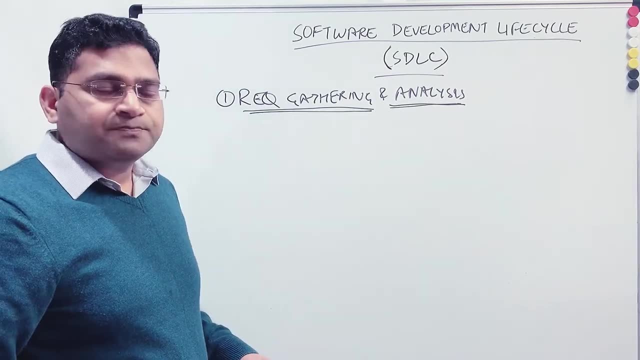 Because of that, you might not be able to fulfill those requirements or not be able to implement those requirements. So in that particular case, what you need to do is you need to basically analyze and understand that, whether those requirement implementation is possible or not, 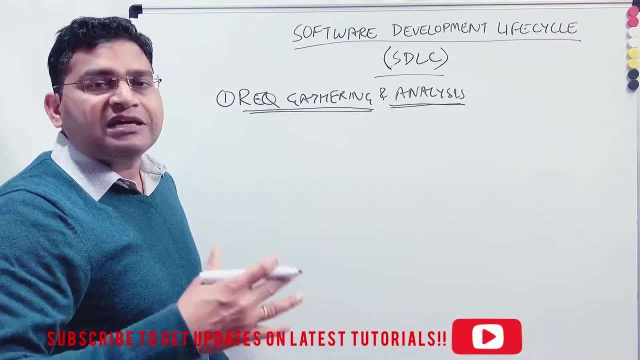 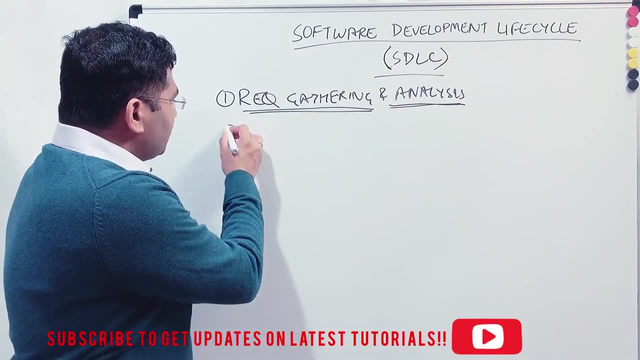 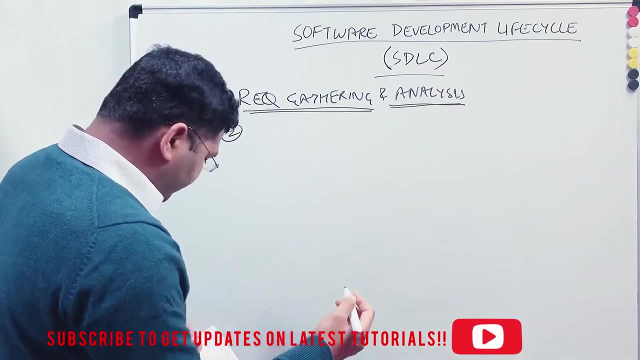 If not, you need to communicate that to the customer about that analysis, and then there will be discussion and updates accordingly to the requirement. OK, so this is about the requirement gathering and analysis phase. This is the first phase of software development lifecycle. The next phase is the design phase. 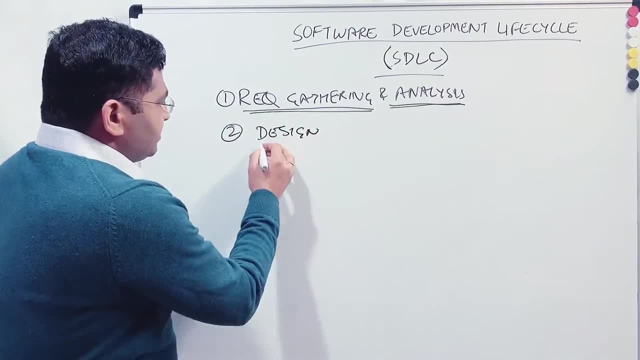 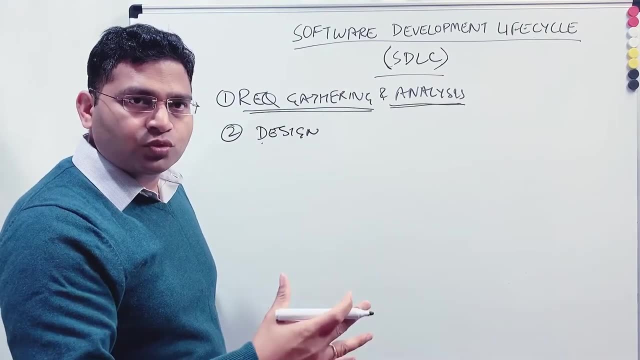 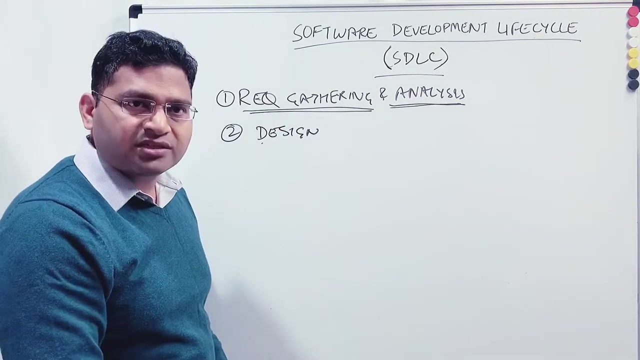 All right What this design phase is all about. So once the requirements are available in the design phase, what the technical architects do is: in the team, you have the requirement And based on those requirements, you want to basically lay the foundation of how the software will be built. 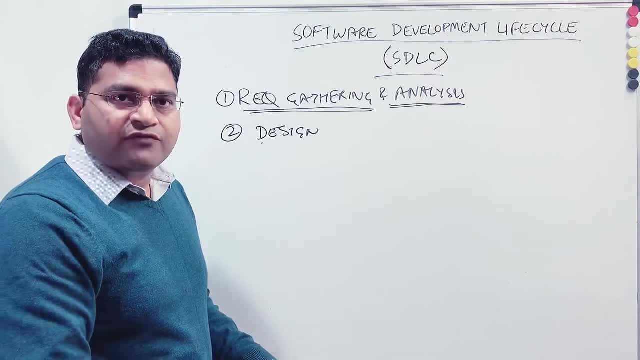 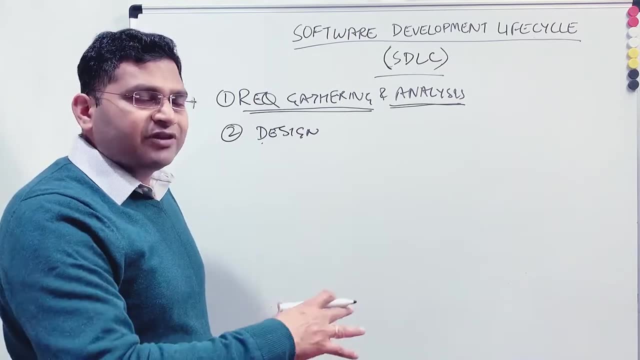 Right. So say, for example, you want to build a house, OK, so the first thing you do is you design how you want to build. You don't start building the house without having a design and understanding how the house will look like. 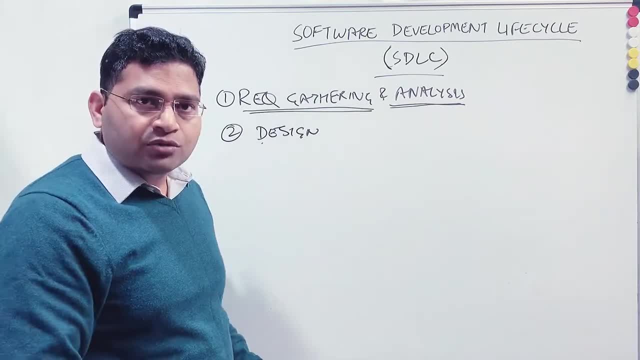 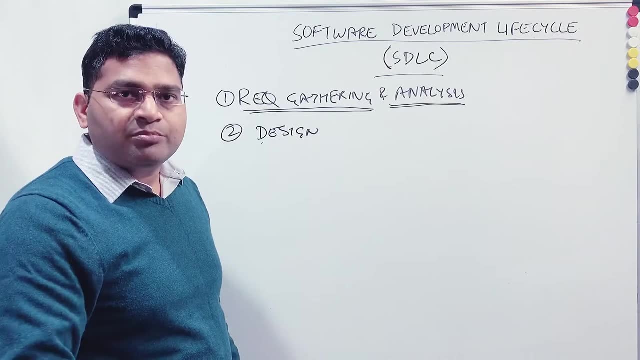 So if a customer said that I want to, you know three rooms in my house, two bathrooms, you know two kitchen, living room. So all those things need to be designed properly first and shown to the customer and clarified from the customer. 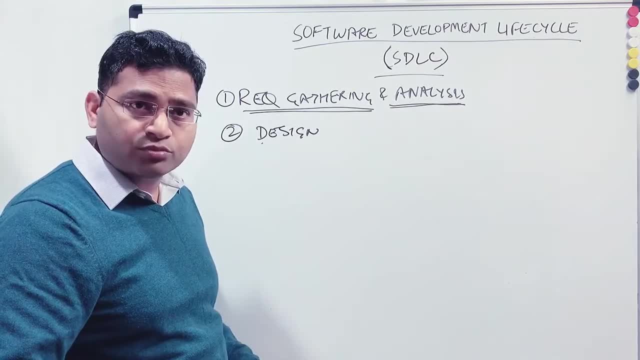 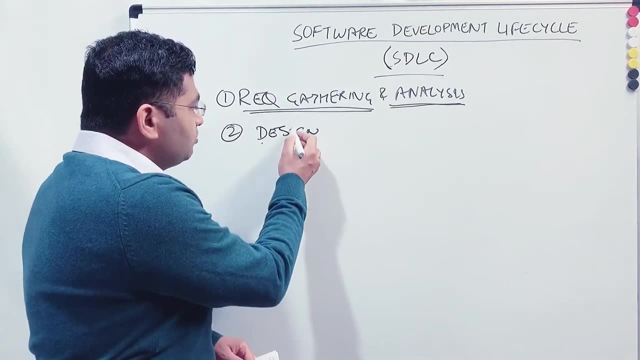 Is this how you want to? you know? Is this where you want to your room to be? is this where you want your kitchen to be right? so same is true with the software: you need to basically first design based on what you have got gathered as the requirement. 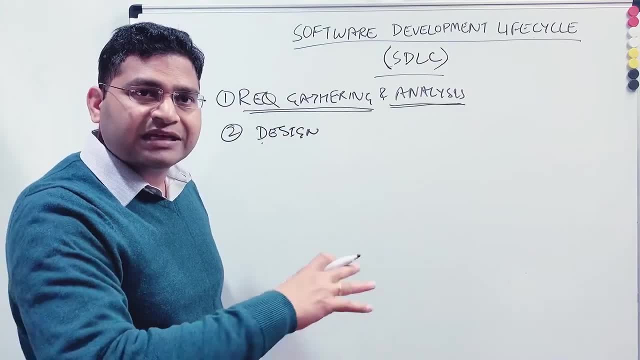 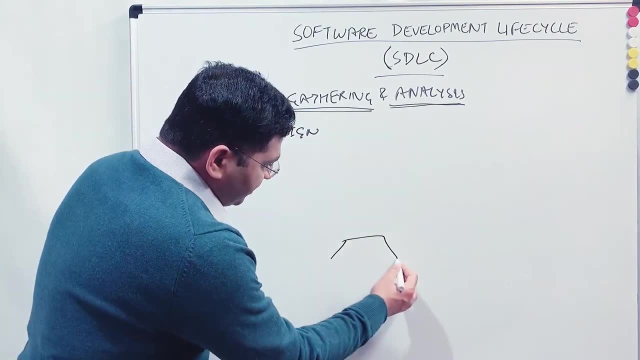 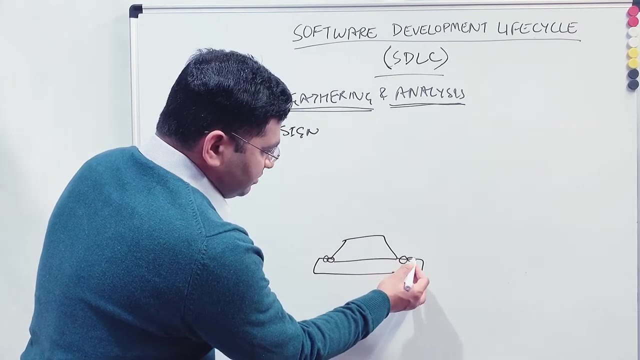 and then analyze with the customer the design that that's what exactly he's want, he wants or she wants. so similar is the case, like the car case. so i have the car. a customer asked to you know, build a car with four wheels and i have put four wheels here right. so this is not fit for you. so i 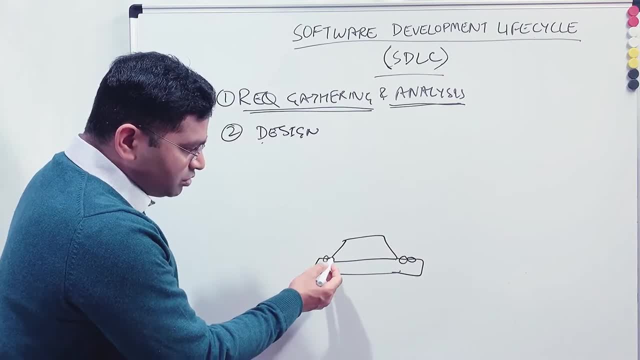 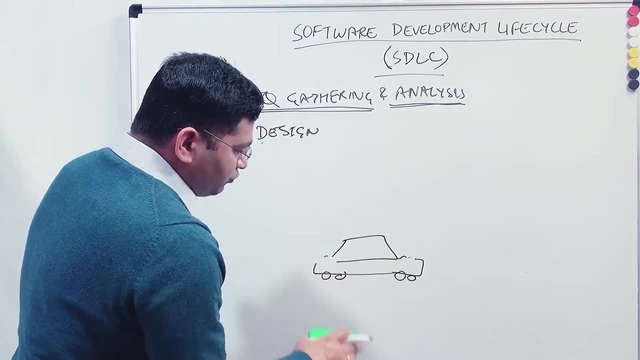 need to basically have the design and show it to customer, whether you want wheels here or whether you want wheels here, right. so customer will say no, no, no, this is not i want. this car is not going to move, right so i want a car that moves. so this is how you clarify the requirement with the customer. 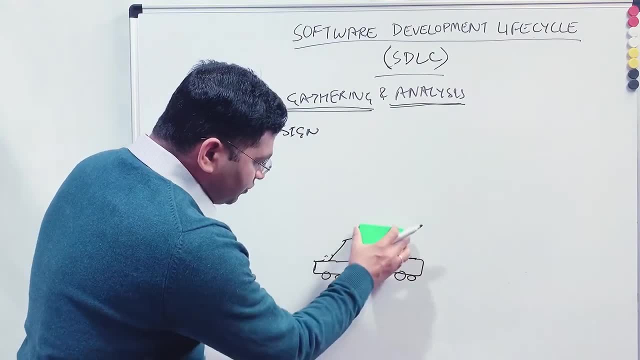 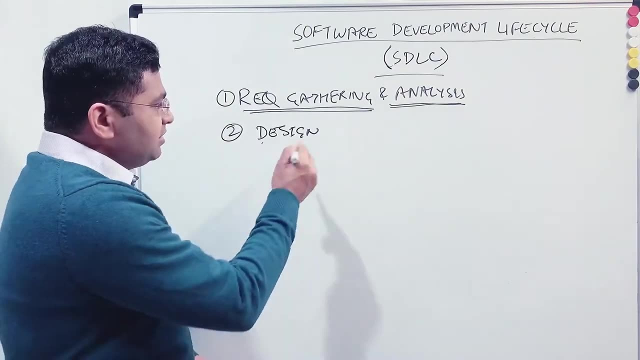 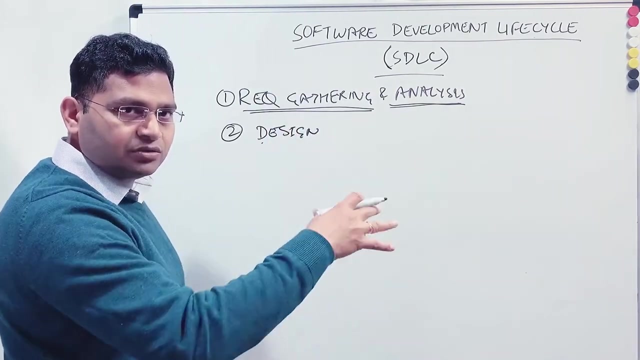 okay. so in the design you design how the overall software is going to. you know what the design will look like, so technical architects do it, and then this is what the design phase is, and in design there are different phases as well. so high level design, low level design. 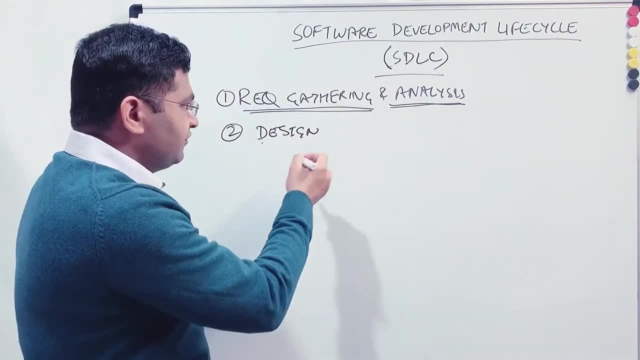 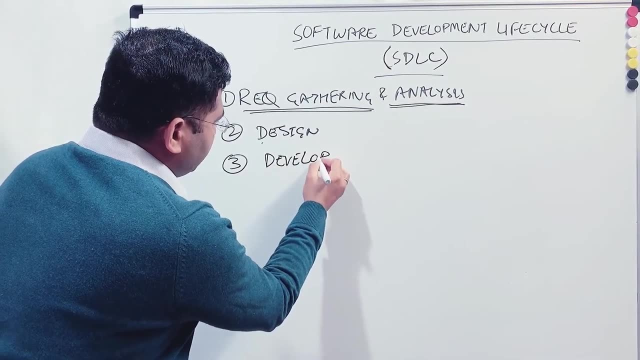 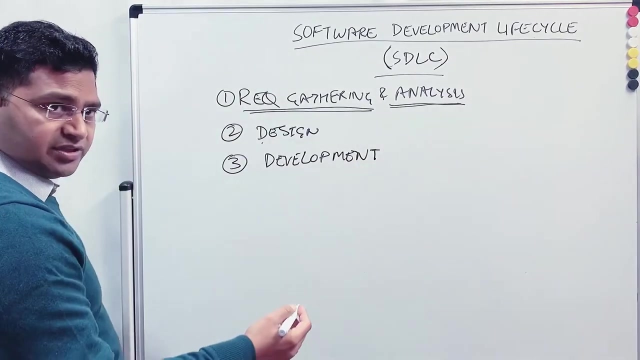 that is within the design phase. so that's the second phase. third phase is develop. now, what happens in develop is so development. so development phase is actually the coding phase, right? so once you have the design ready and you know what you are going to build, then you start. 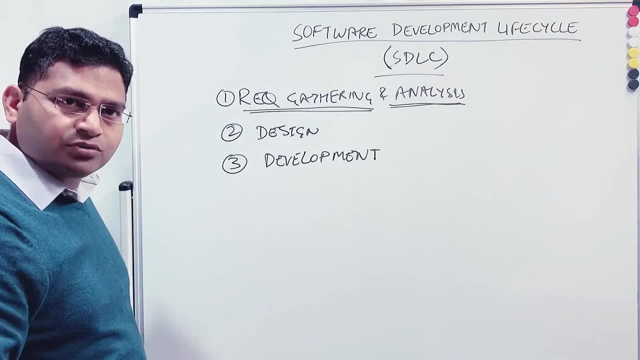 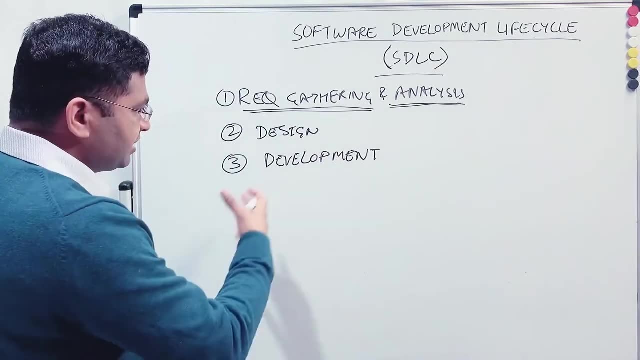 the development work or you start building the house right. so you have the design, you have the foundation laid and then you know you start putting the bricks. and same is the case with the software. so once the design is ready, the next phase is the development or coding phase, wherein 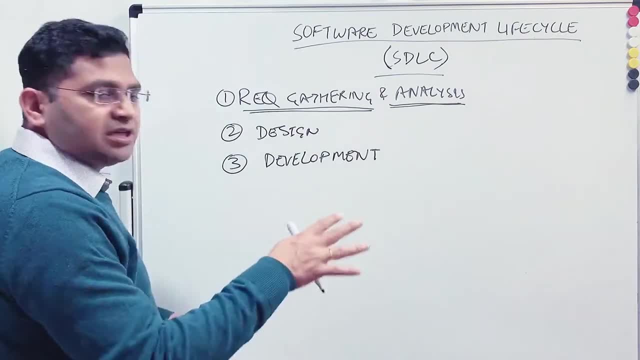 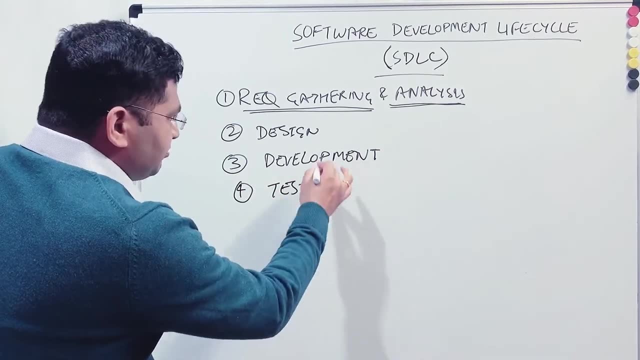 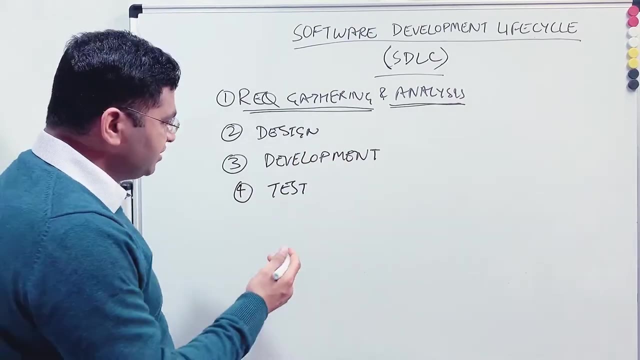 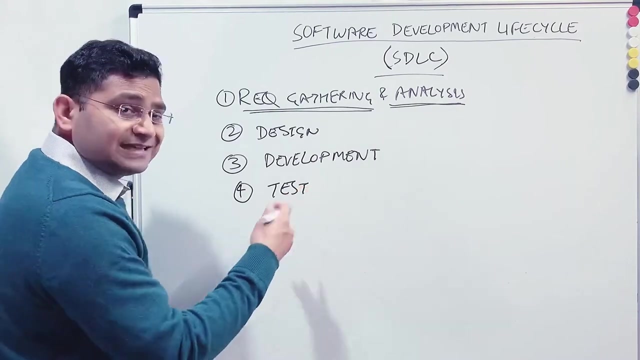 the development team will start writing the code to implement those requirements. okay, the fourth phase is the test. okay, so, once the development is done and a development team has, you know, created certain features or developed certain features, they will provide those features or they'll deploy those features into the test environment for the testers to test. okay, now, if you're, you will be. 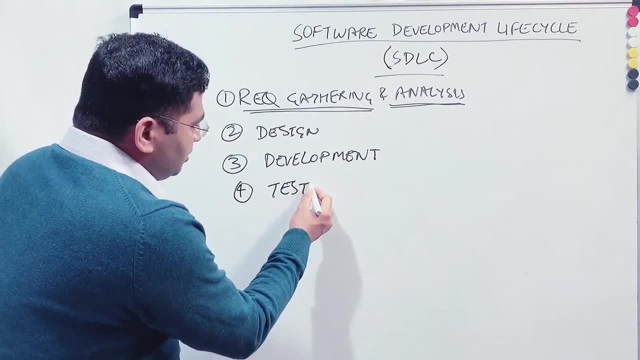 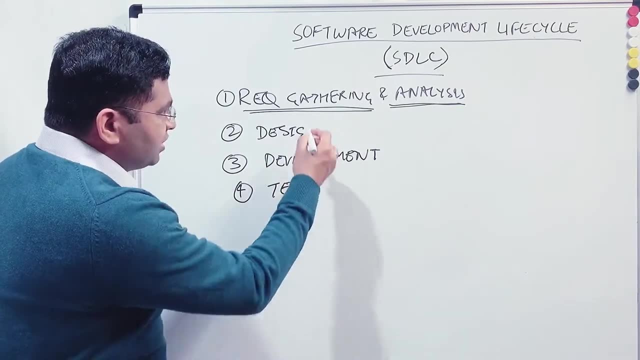 working as a test tester within team, you will go to that particular you know test environment and launch the application or the application and you will be able to test the application. and you will be able to test the application and verify that whatever features or whatever requirements are. 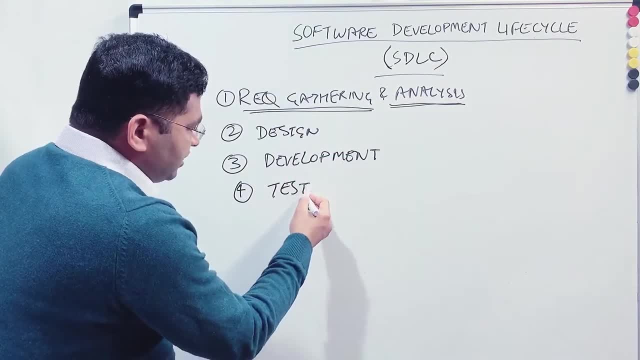 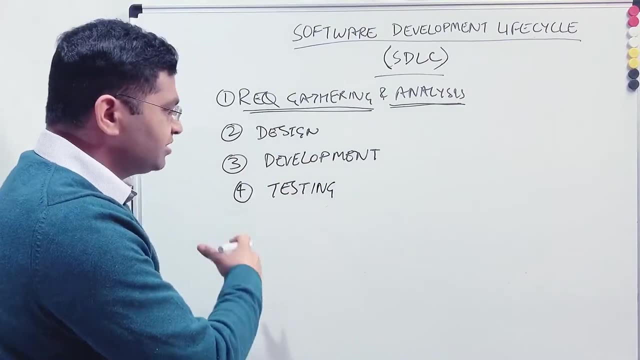 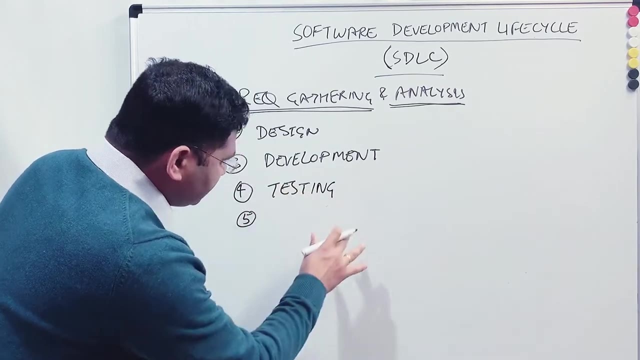 being built in this particular release. they are working as expected, right? so this is the testing phase. so in testing phase you do the testing work for the application or the app. okay, then, after the testing is successful, everything is fine and stakeholders have agreed to release the software. 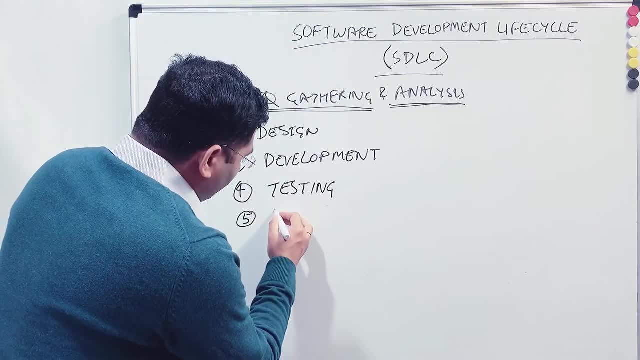 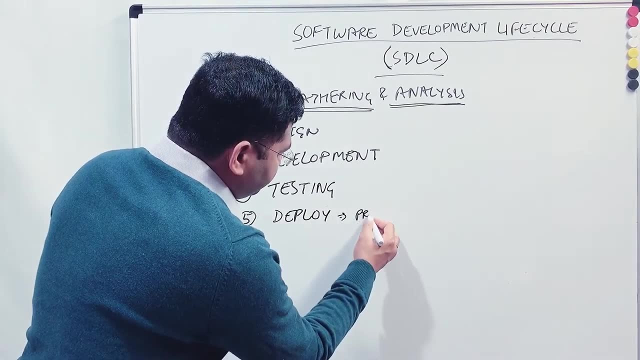 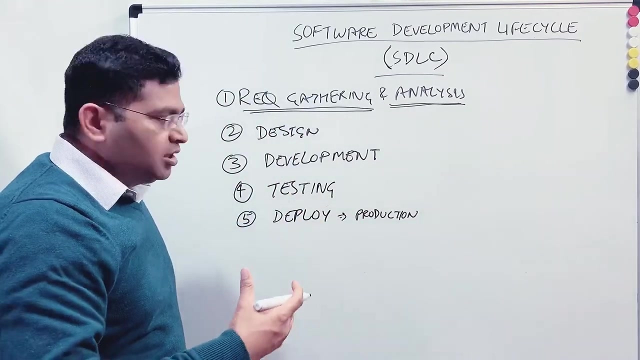 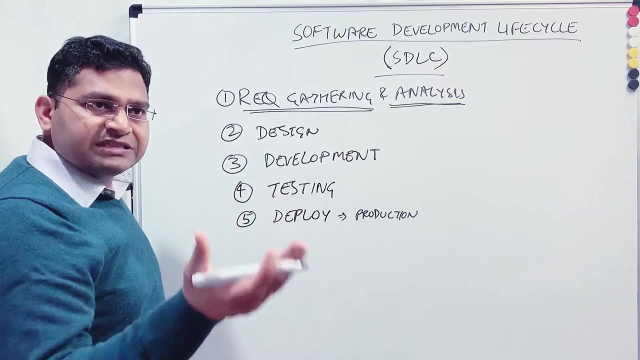 the next phase is to basically deploy. right, what does deploy mean? so deploy means deploying to production, so you won't be having all the code into the testing right. you have to basically move it to production where the customer can access. or if it is for the public, you say, for example, gmail is the application which is used by. 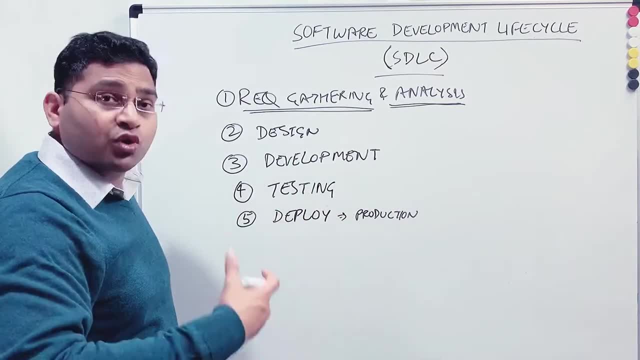 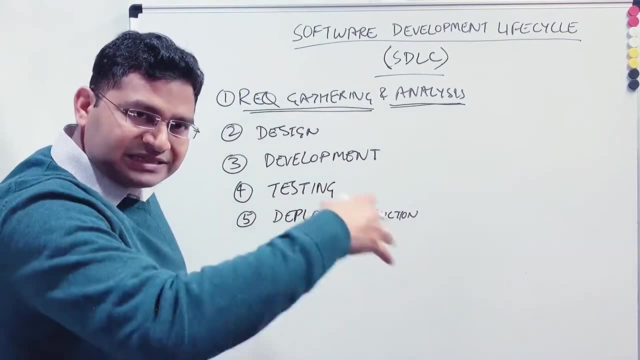 everyone right, or all the public, whosoever has the gmail account or wants to create a gmail account. now, if gmail google would have done that. if the gmail app is not being used to create an account, developed and just kept it there in their testing environment and not available over the internet. 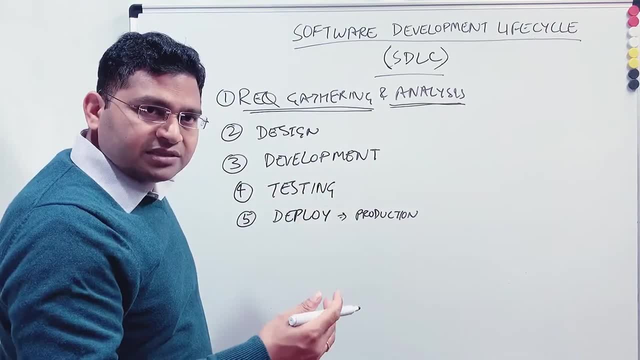 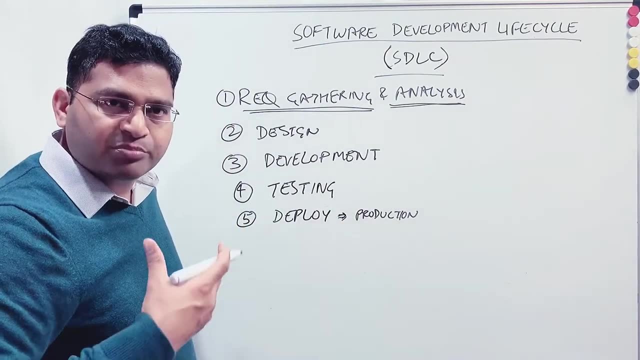 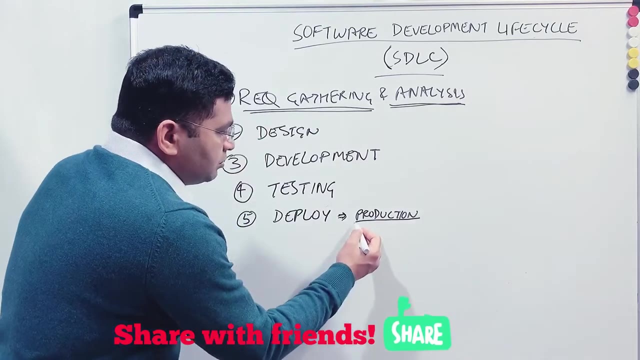 then that's just within their organization. it's not available to the public. now, if it wants the customer for gmail, are the people like you and me right? so they have to move it to the production over the internet, and this is what deployment is. so in the deployment they move the code to. 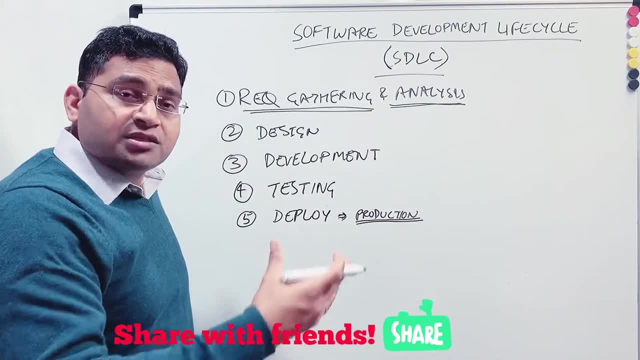 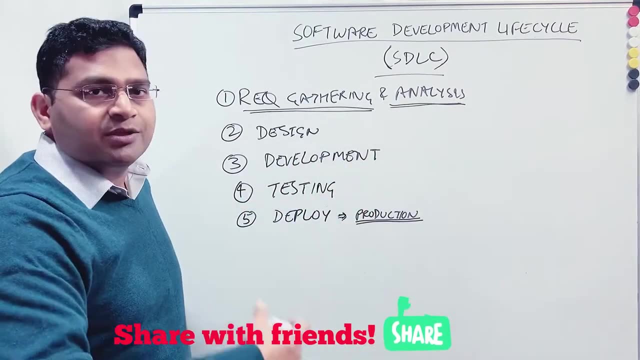 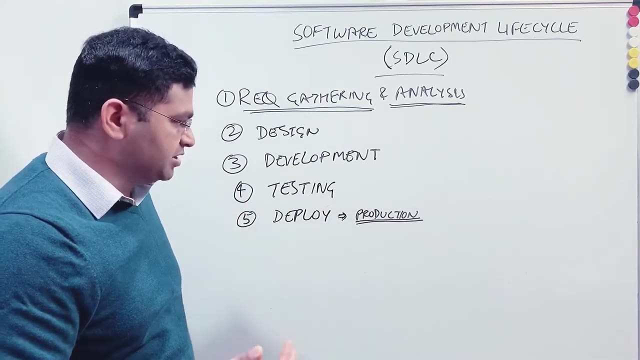 the production and make it available to the relevant customer for whom that software is being built. so in gmail case, it is for us and that is why it is, you know, deployed in the data centers, or the whole code, and it is available over the internet for us to access the gmail emails all. 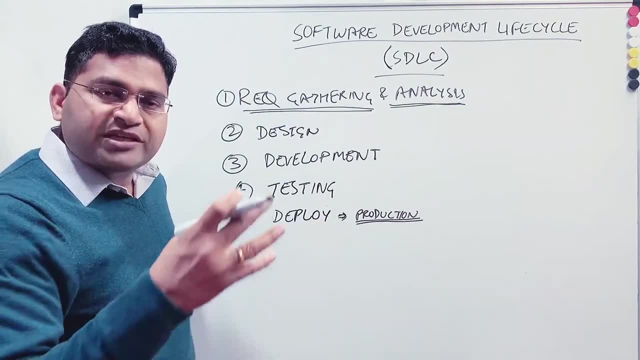 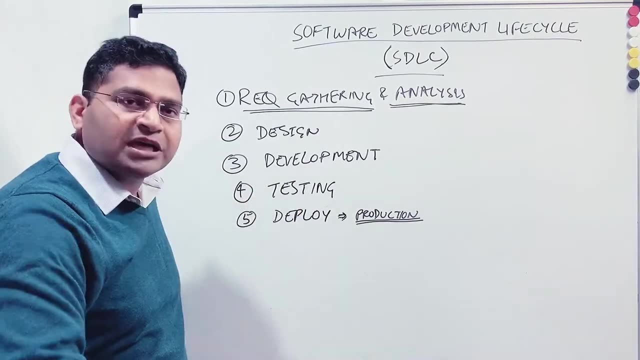 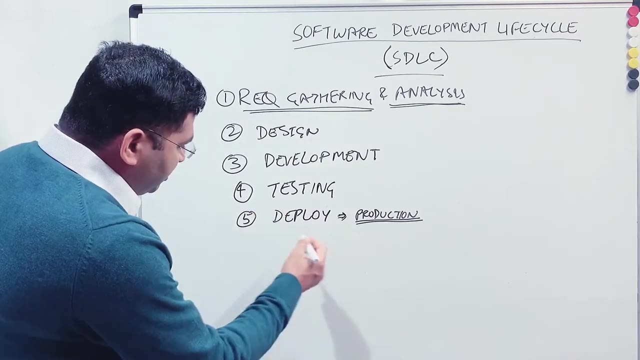 right. so in the deployment phase the actual code is being deployed for the customers who are going to use it. it might be a set of customers or it might be the wider public, you all right. so it depends what the context is of that particular software. so after the deployment, 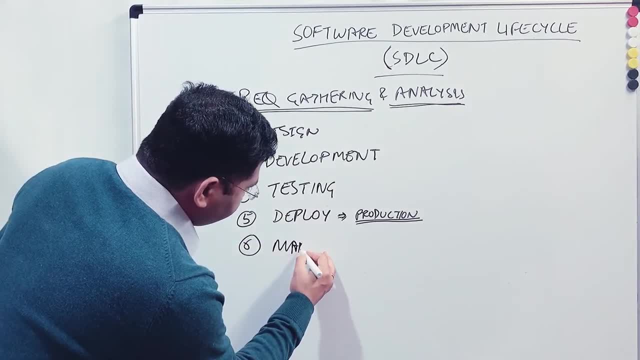 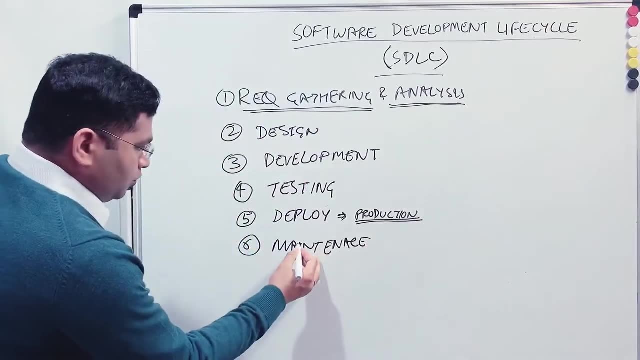 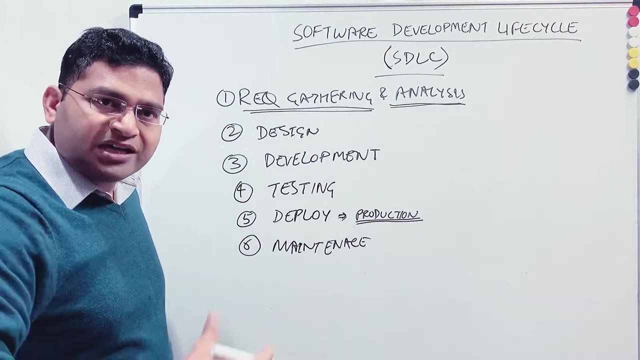 phase. the next phase is the maintenance. all right, so in maintenance phase, once the deployment happens okay in the production, the software needs to be maintained, right? so, for example, you buy a car, you bring it, it's a new car. after every six months you have to service it. 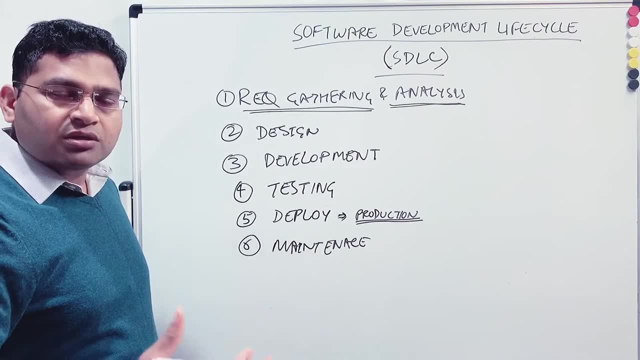 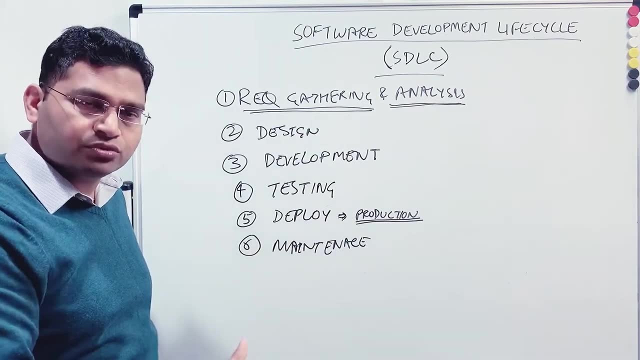 right. so it is required, because if you want to use the car without any issues, you have to basically take care of it, you have to maintain and you have to see that there are no issues or there are there are. every functionality or machinery is working as expected. similarly, in 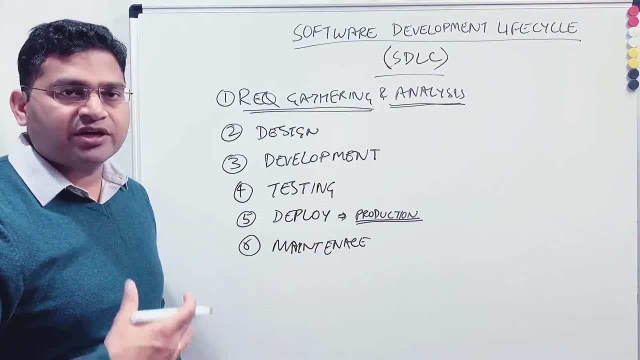 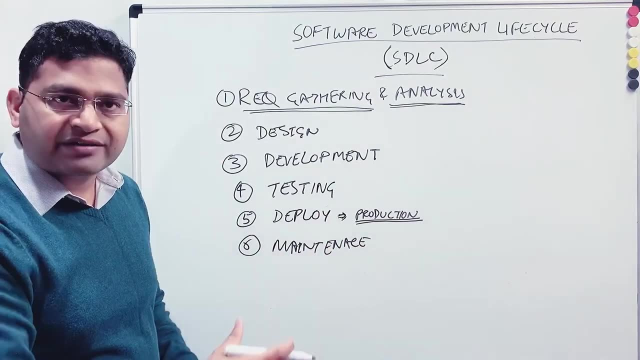 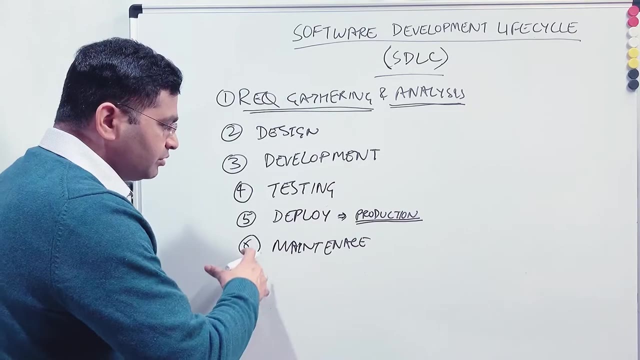 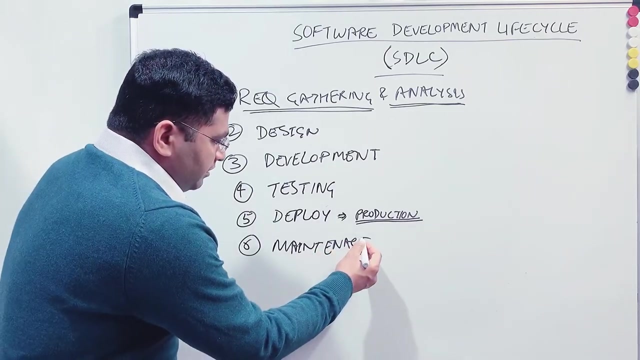 software. you have to basically ensure that you do that maintenance or regular maintenance for the software so that it is not, it doesn't crash. so say, for example, the software due to, you know, hardware issues or there might be, you know, issues within the software itself. so, as we have already understood about the seven principles of software testing, so 100 testing- 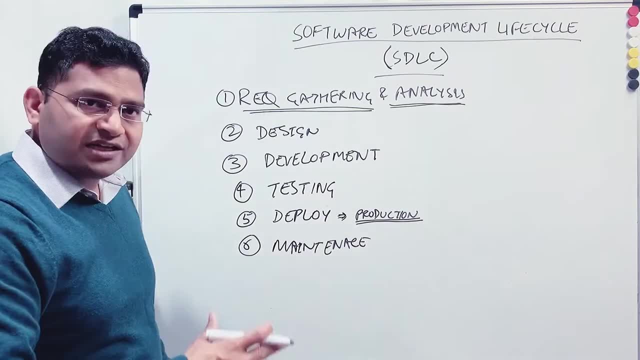 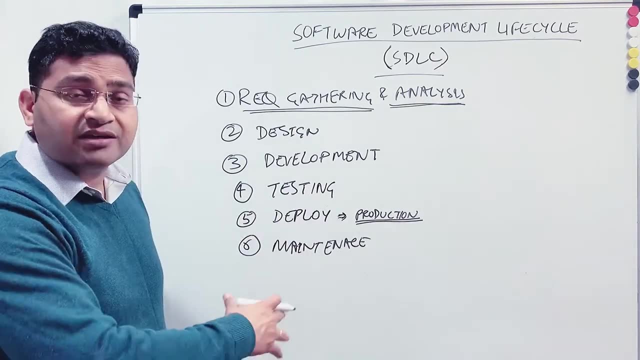 is not possible and even though if you still can't find any more issues in your software, it doesn't mean that the software that deployed, that is deployed in the production, is 100 defect free right. so you can't say that. so in maintenance phase what happens is you basically 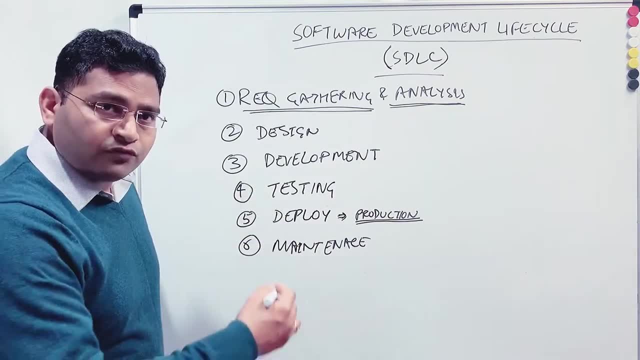 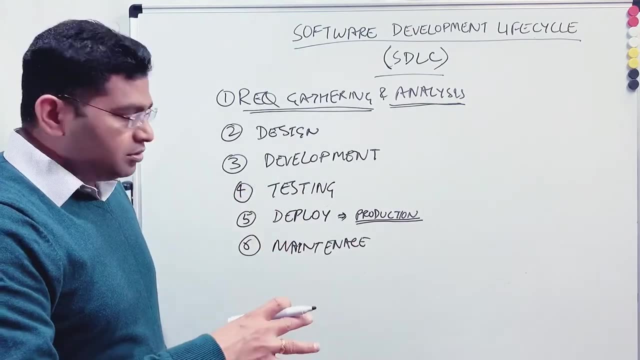 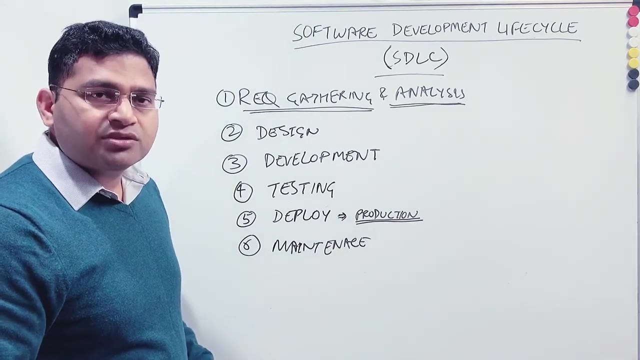 regularly maintain the software and you also fix any of the production issues that come through right. so once the software is in the maintenance, you keep a watch on what all issues are being reported by the customers and if there are critical issues or any issues that are being. 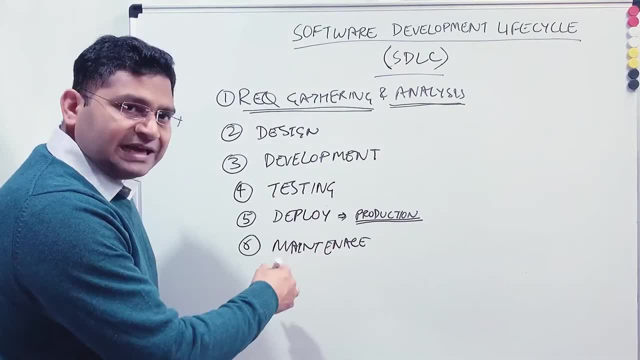 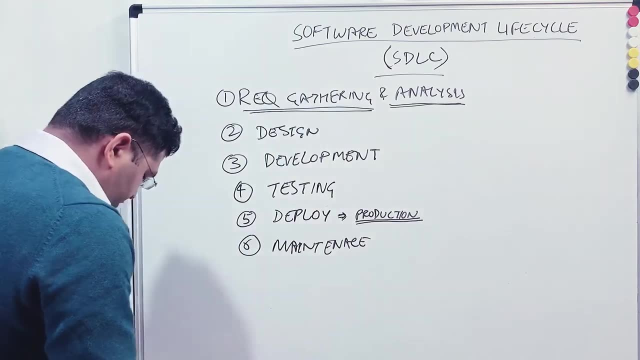 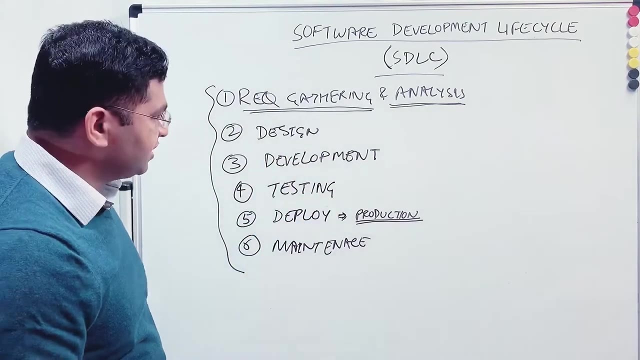 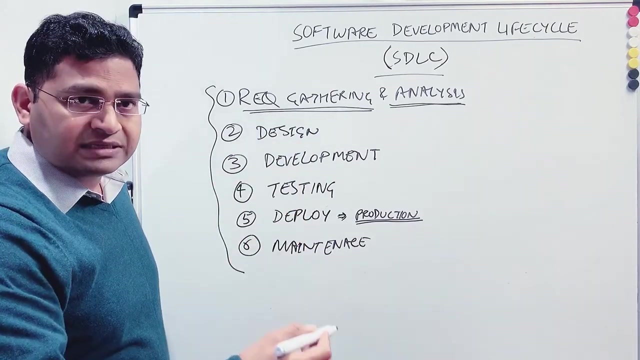 reported by the customer, they are being fixed and redeployed in the production. so this is what all happens into the maintenance phase, right? so these are the key six. so basically six phases of software development life cycle, and you need to understand the software development life cycle before you understand software testing life cycle. 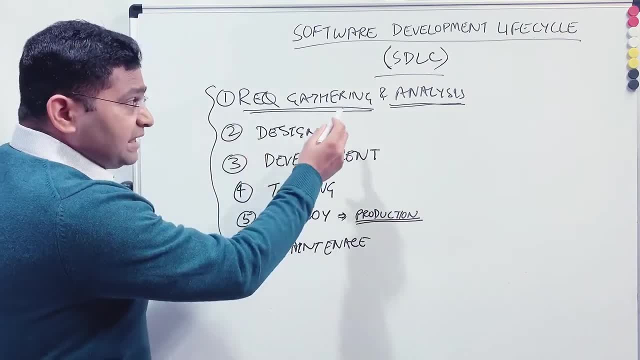 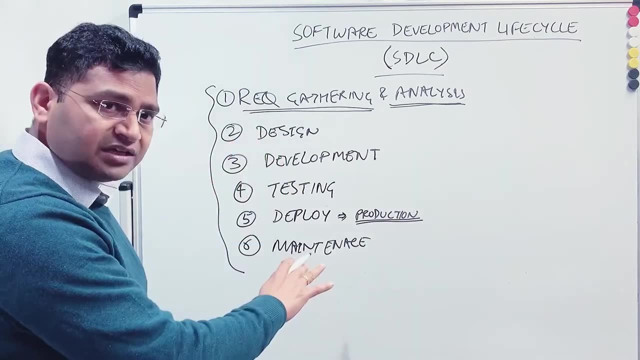 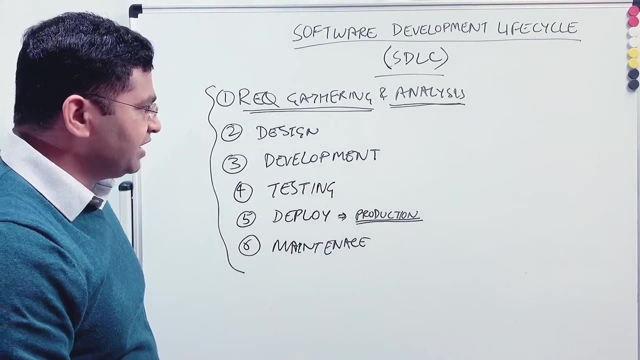 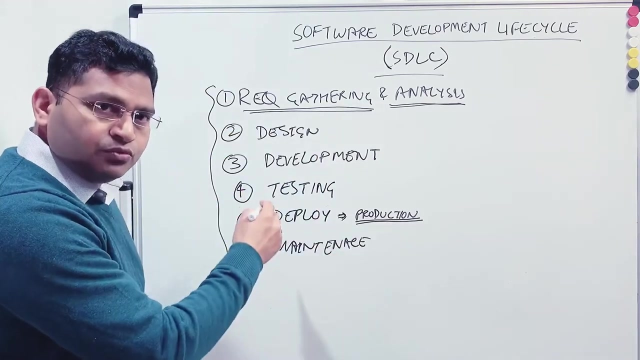 in the next tutorial that i'll cover right. so, requirement gathering and analysis, design, development, testing, deploy and maintenance. very simple, it's a phase or a life cycle that any development team will follow to develop any software or application. right now, these phases- this is, uh, you know, will remain true for waterfall- 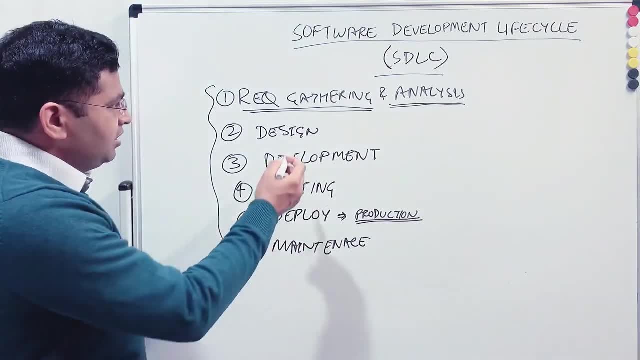 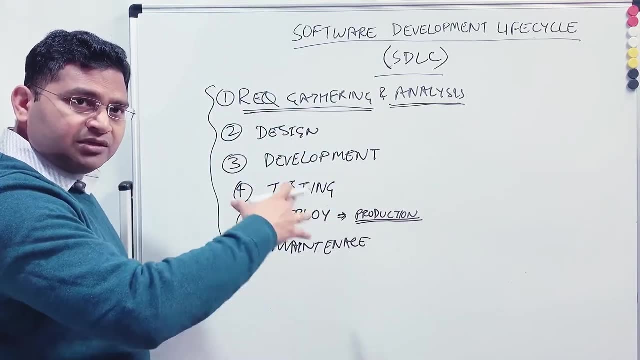 for remodel, for and even for agile right. so in agile, uh, you know, you will have the requirement gathering. so this is this won't happen in each and every sprint, but it will happen in, you know, say, for example, two to three months, or in in a one increment, a program increment. so there will 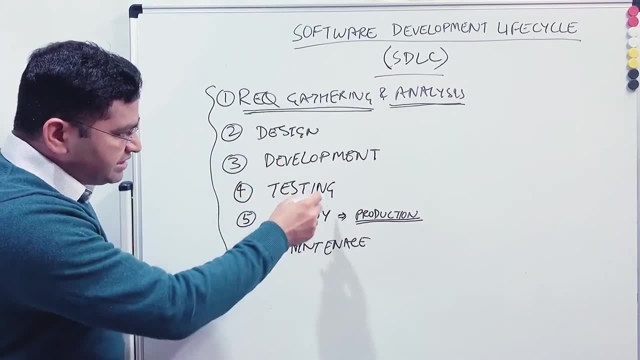 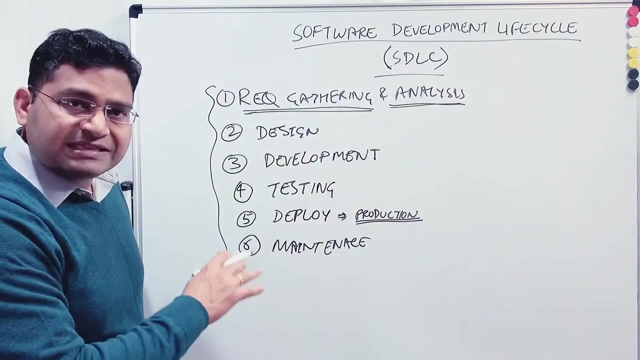 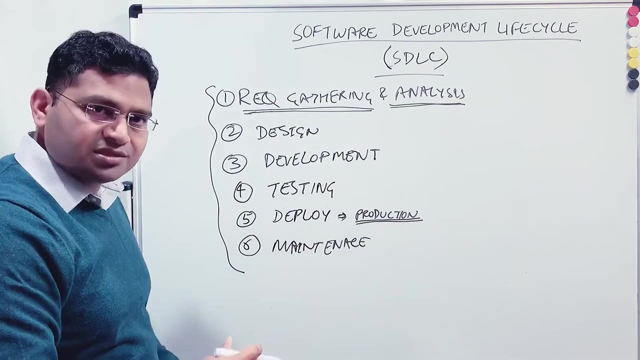 be requirement gathering phase and then design development testing testing will happen. design development testing happens in very short iterations- two to four week cycle, but phases are still same, so phases will still be there. the only difference which happens between these development approaches is the timeline that you follow in waterfall approach. 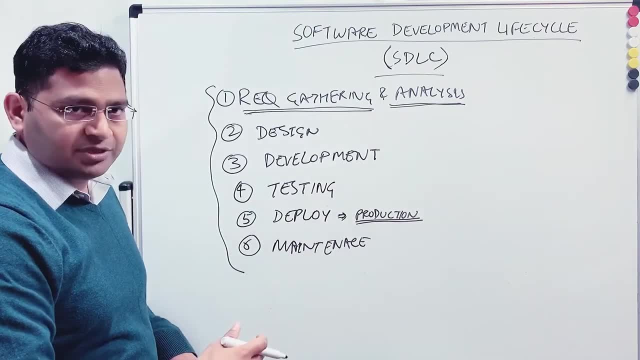 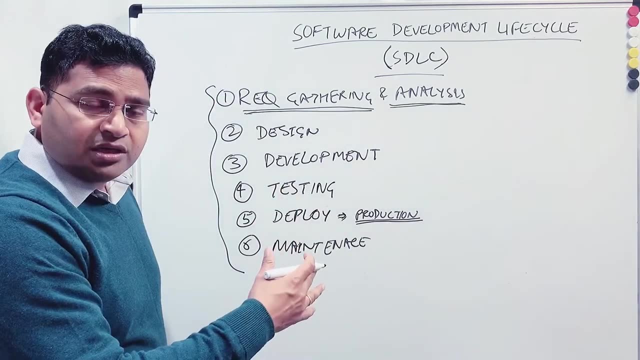 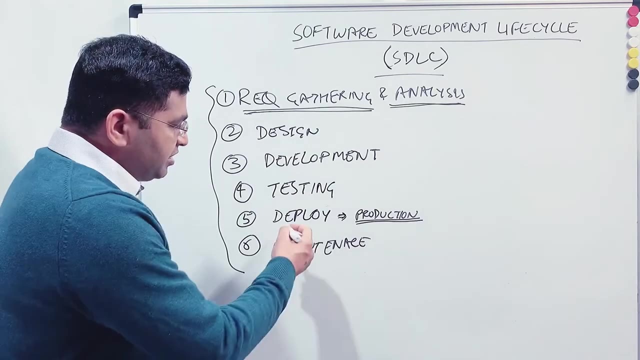 it will be longer timelines in agile. it will be smaller timelines in agile. maintenance, uh, you know like deployment and maintenance or deployment to production uh, can happen every month, okay. so it depends how the organization wants to deploy to the production, okay, but in waterfall it was usually like six months to one year, so it depended, uh, how the organization wants to deploy. 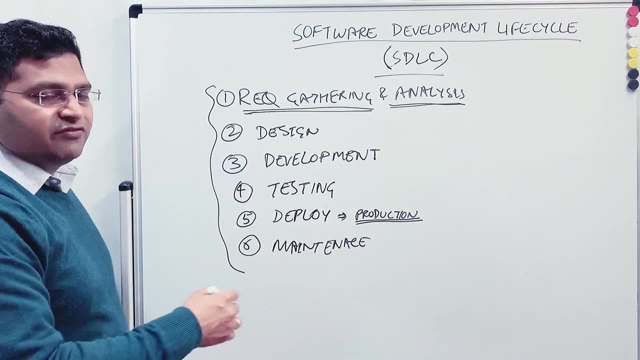 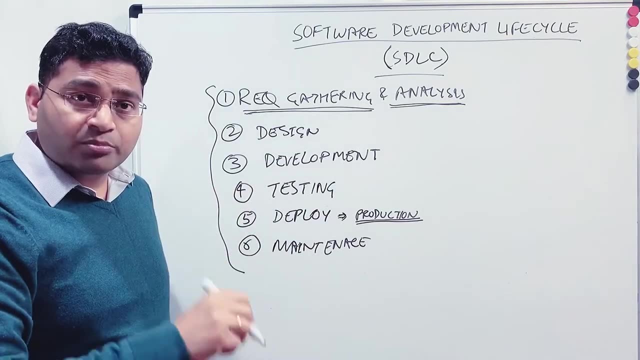 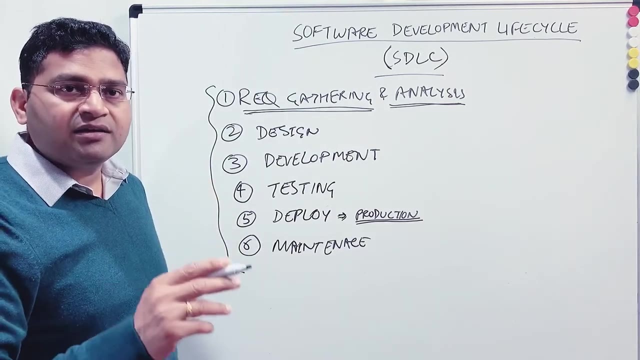 to production waterfall approach, right? so this is the basics of a development life cycle. um, understand it very well. if there are any doubts, please comment in the comment section and i'll clarify all those doubts so that you are good enough to go ahead and explain it to any interviewer in the software testing interview. so that's all for this tutorial. please do share and subscribe and thank you very much for watching.